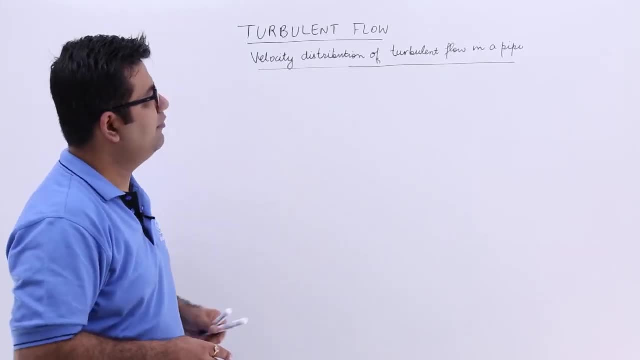 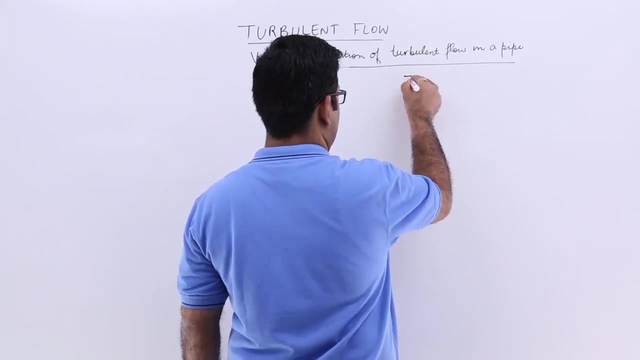 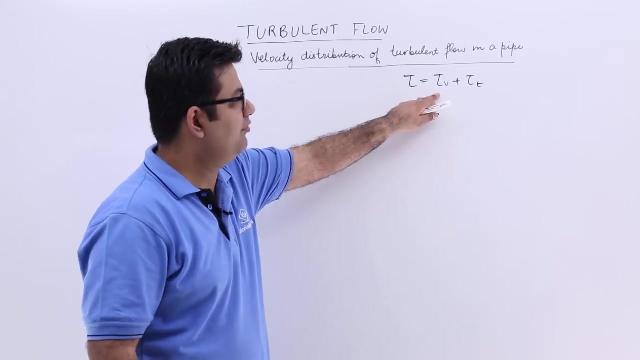 Now let's talk about the velocity distribution of turbulent flow in a pipe. Now, if you talk about the shear stress in a turbulent flow, that is, tau is equal to tau v plus tau t. That is the sum of the shear stress due to viscosity plus the shear stress due to turbulence. 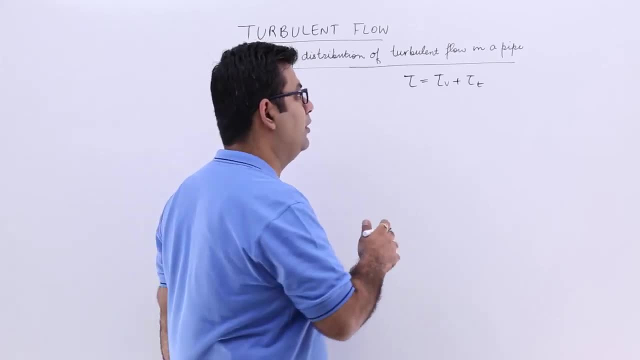 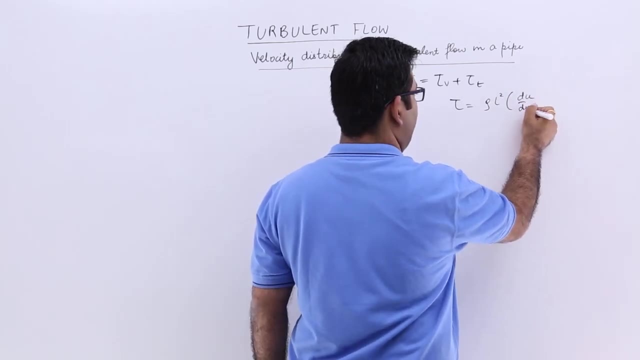 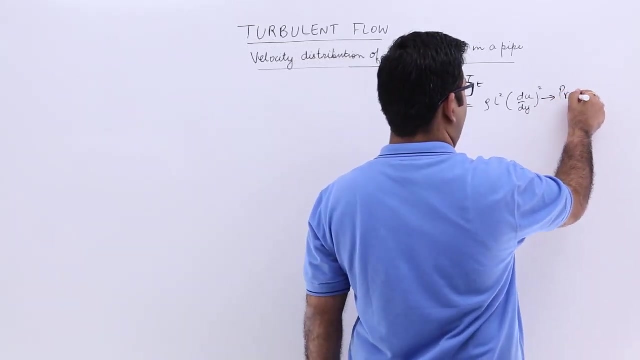 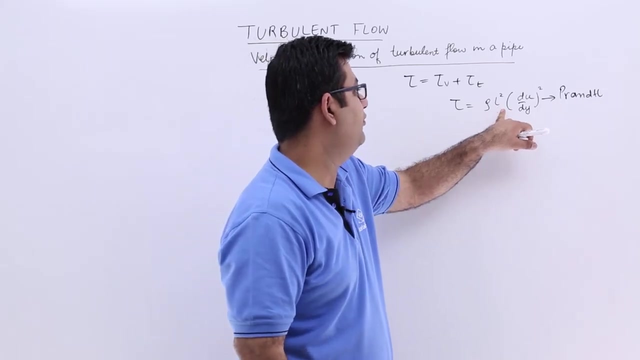 Now the distribution of the shear stress in a turbulent flow is given as rho into l square, into du upon dy whole square. Now this is the relation which was given by a parental Alright. Now this means that if I know the value of l and if I know the value of y, I can find out the value of tau. Okay, 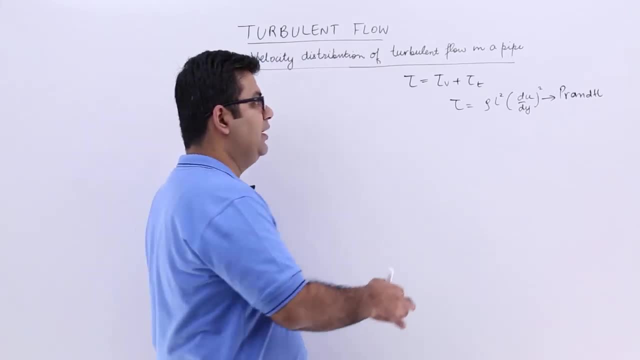 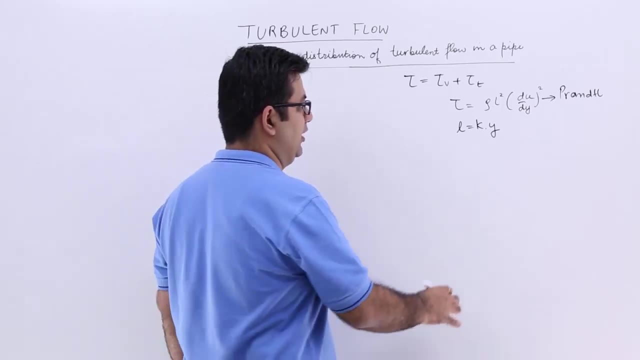 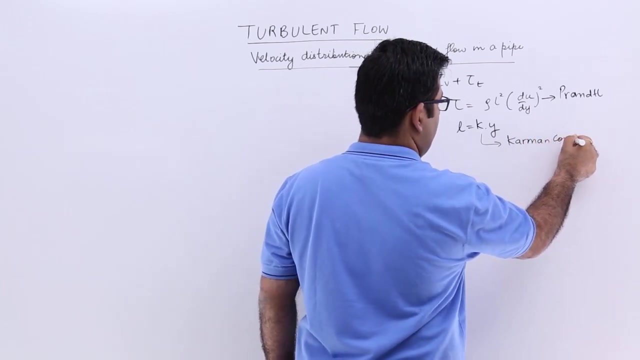 Again, there was a relation which was given by a parental between l and y, that is, l is equal to k into y. Okay, So k is a constant which is called the Kármán constant, and this value is equal to 0.4.. Okay. 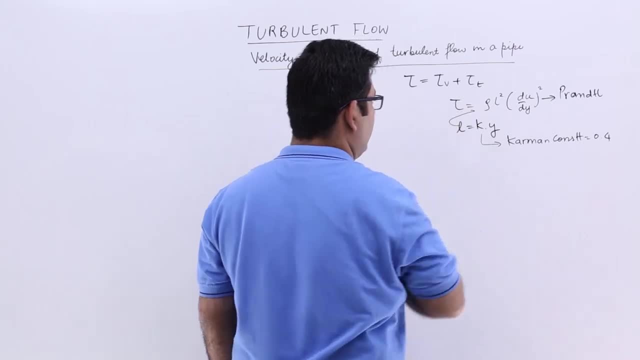 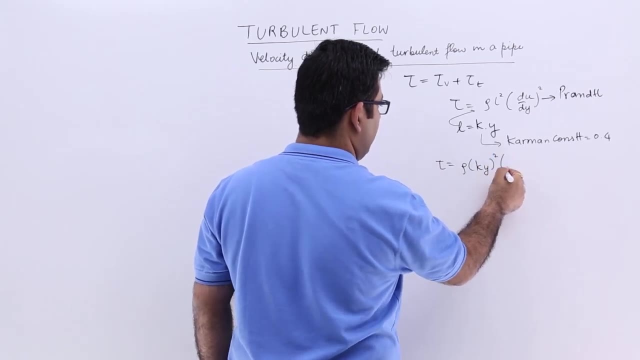 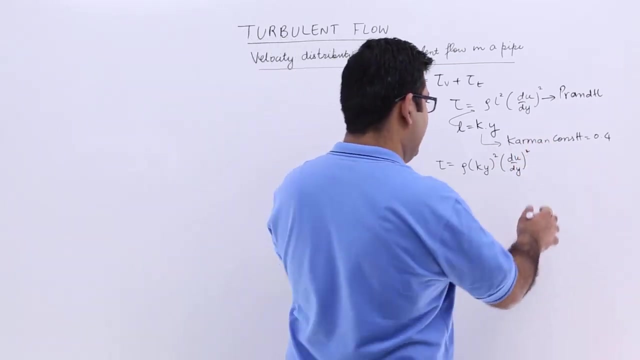 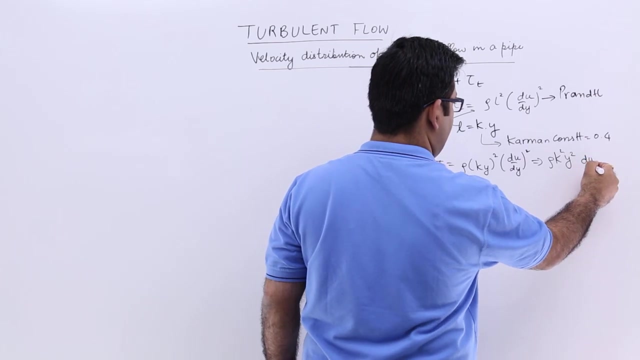 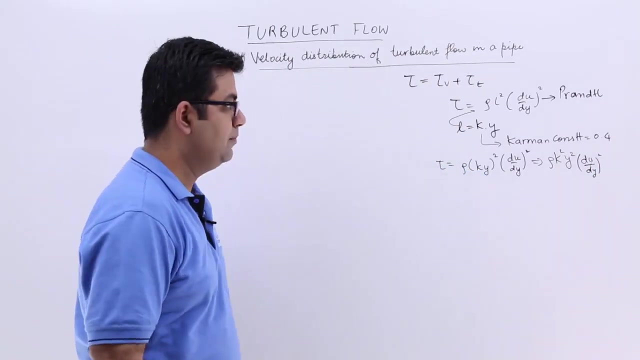 So if I put the value of l back into this equation, I will get: tau is equal to rho rotor into k, into y whole square, into du upon dy whole square, Okay. And this can be again rewritten as rho into k square, into y square, into du upon dy whole square, Okay. 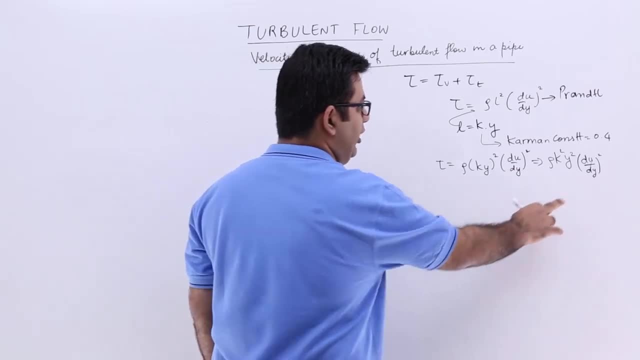 Now, from this equation, find out the value of du upon dy. okay, So the value of tau is equal to tau t by kéu divided by tau y. times dv over tau x, statist third over tau y. This is the definition which, once coming out, So the solution was again a relationship where we are talking about breaking the current in terms of limit of Teus and this increase of value of tau ratio and winner, the future of the probably coughing process, always entity which is terminating and doing an operation which has this: 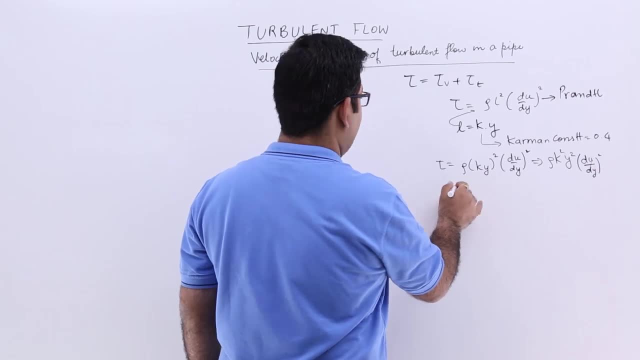 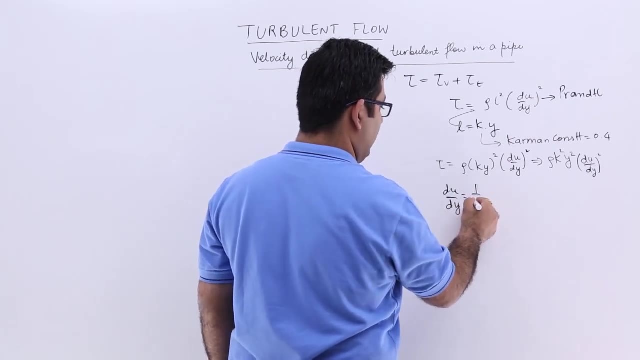 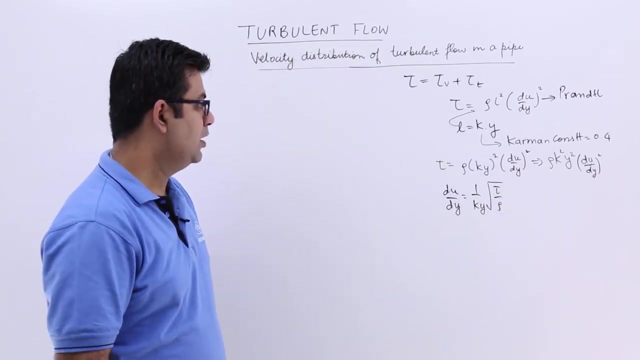 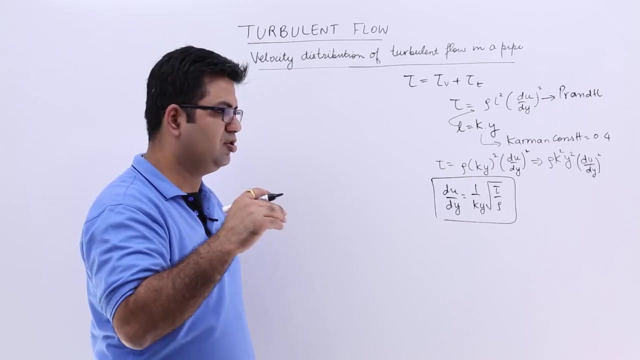 value of du upon dy, because we are interested to find the velocity distribution. so du upon dy will be equal to 1 upon k into y, into tau upon rho, under root. okay, now, if the values of y are very, very small, that is, your flow is almost, you know, near to the boundary. then 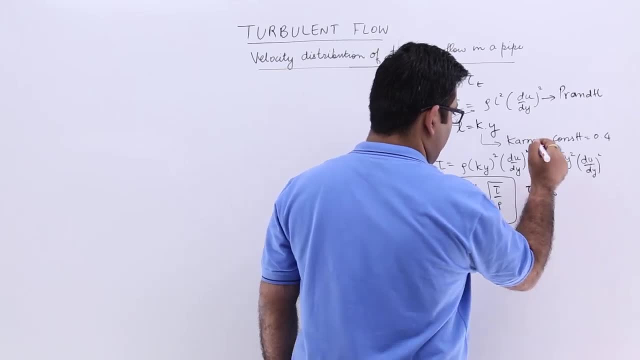 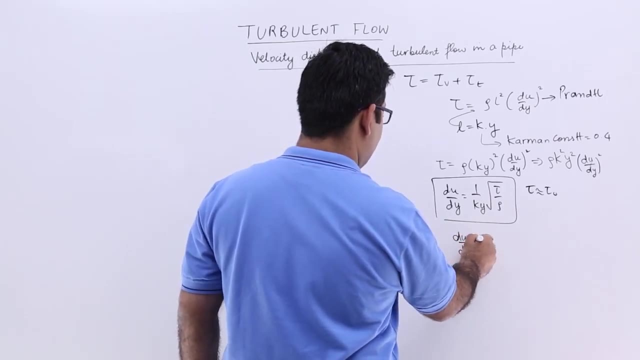 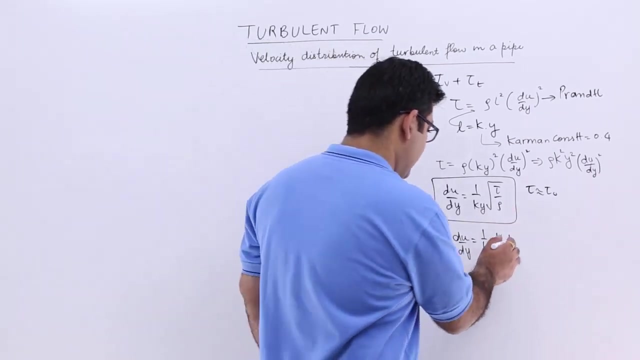 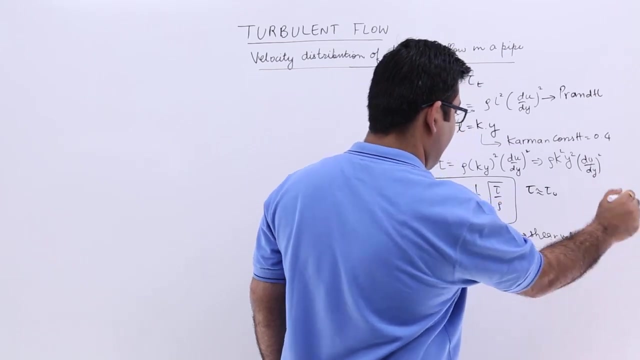 I can say that tau can be almost put equal to tau naught. that's the maximum value. so you will get du upon dy is equal to 1 upon ky into u phi. now what is this? u phi? u phi is called shear velocity. u phi is called shear velocity where u phi is equal to under root. 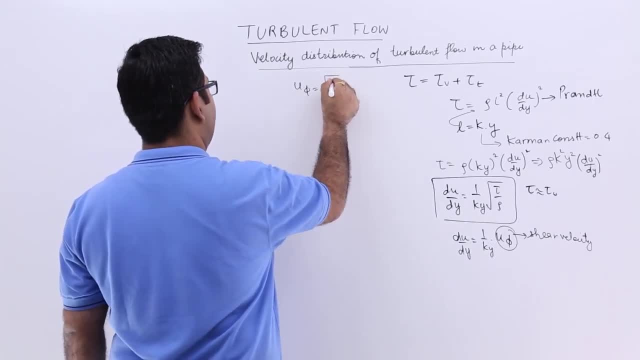 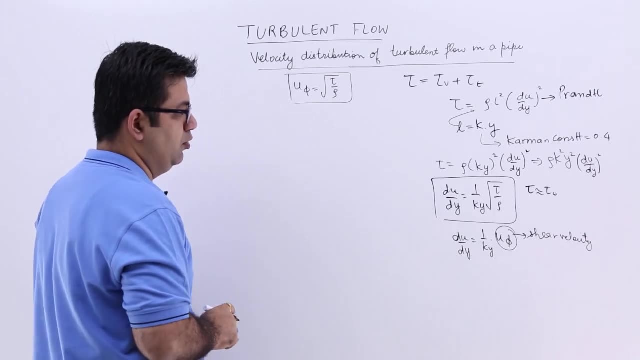 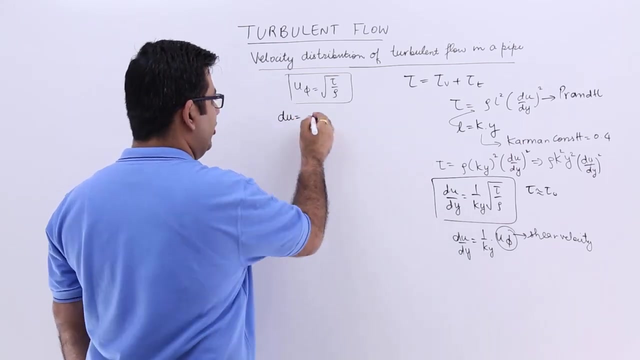 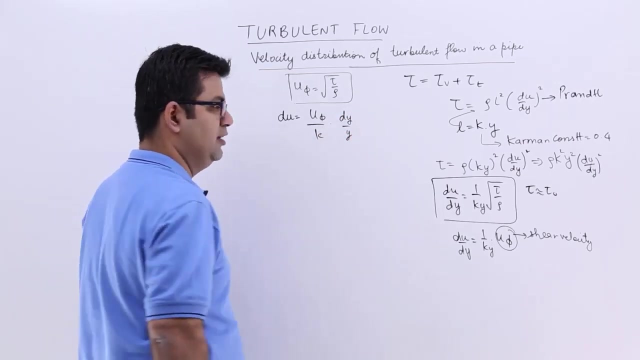 tau upon rho. Okay, So shear velocity is equal to under root tau upon rho. okay, I hope you got this. now let's move forward. so if I write down this equation again so you will get, du is equal to take y on the other side, so you will get u rho upon k into dy upon y. so let's treat. 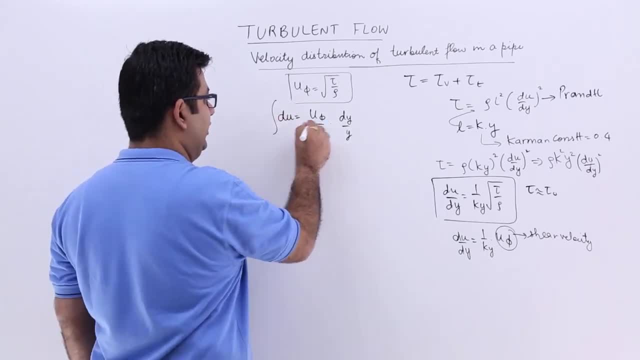 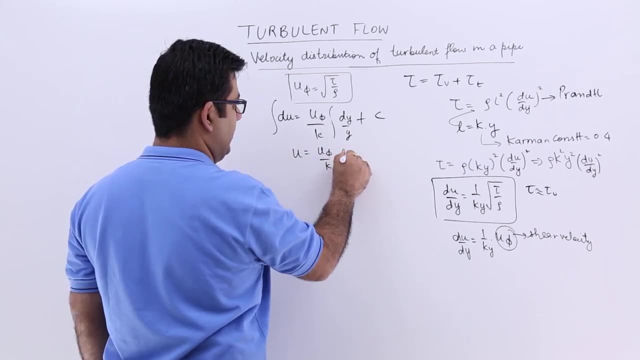 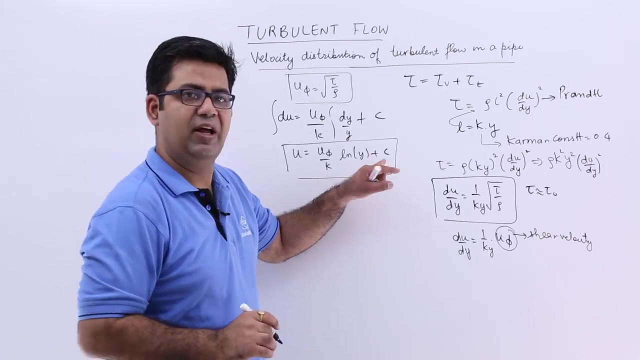 u phi as a constant value and now we can integrate it plus c. You will get: u is equal to u phi by k into log y plus c. that's the value that you will get. now to find out the value of c over here we will have to apply the boundary condition. 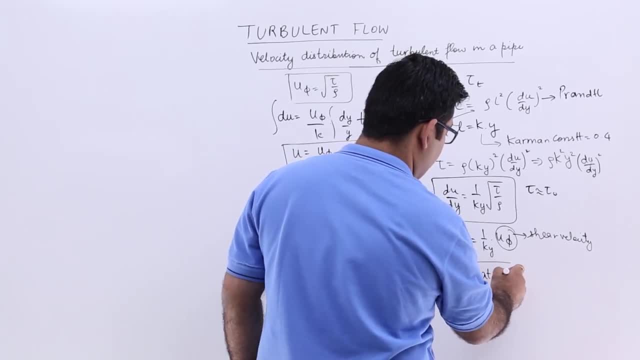 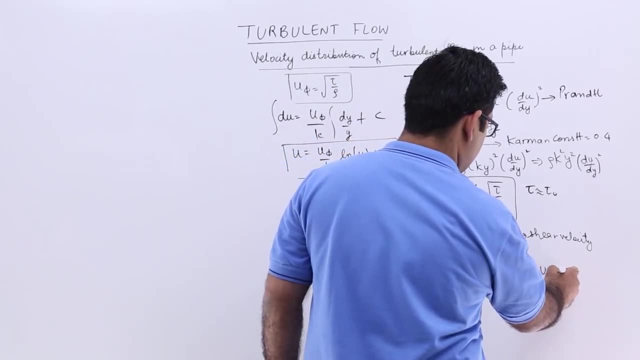 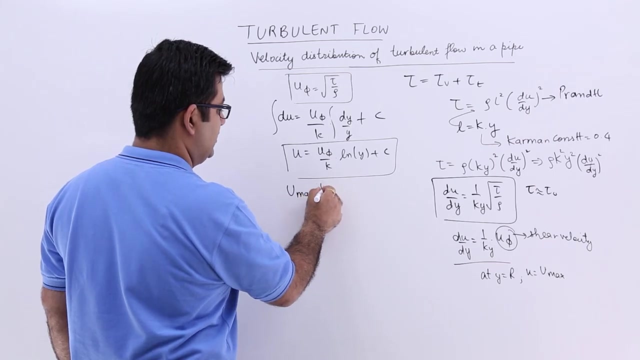 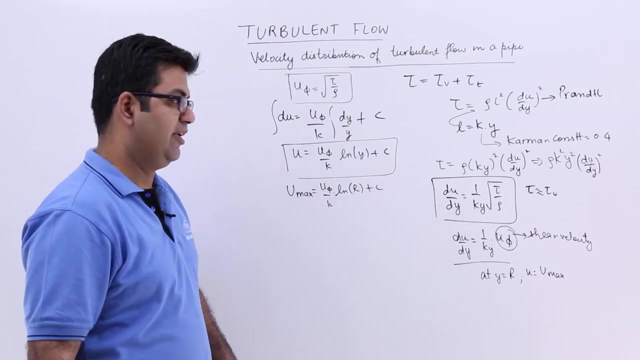 the boundary condition is that at y is equal to radius of the pipe, the velocity becomes the maximum velocity. Okay, Now one comes, becomes that u k becomes y power u and u phi is equal to 5 root 2 by r. right, okay, now here I can say that u will now become u max. this is equal to wish phi. 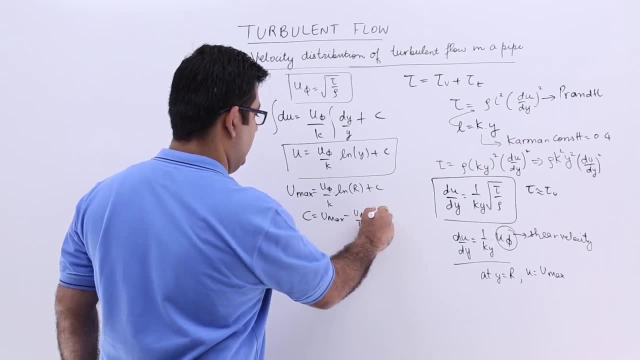 upon k into log r plus c. so find out the value for c from this equation. so it will be equal to u max minus u phi upon k into log r. So let's put the value of c over here, so the value of u will now become u phi upon k into. 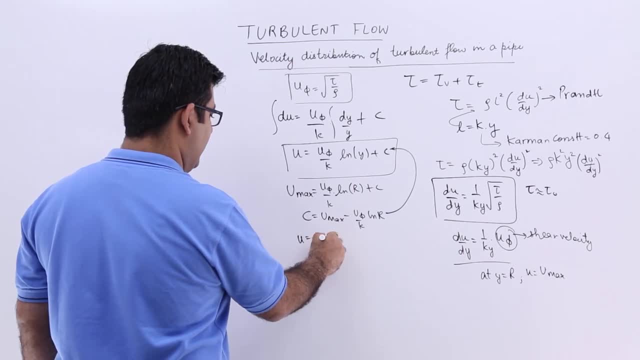 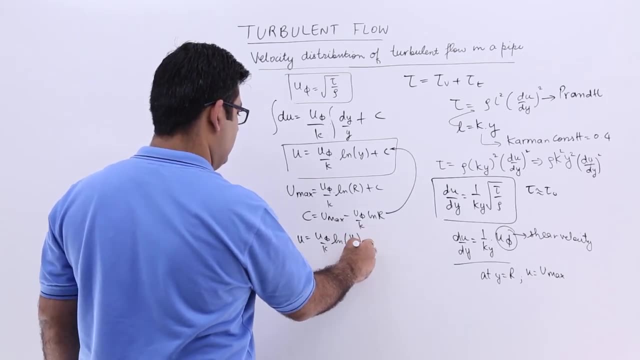 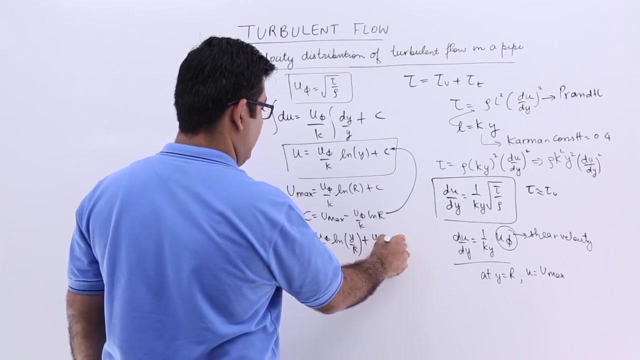 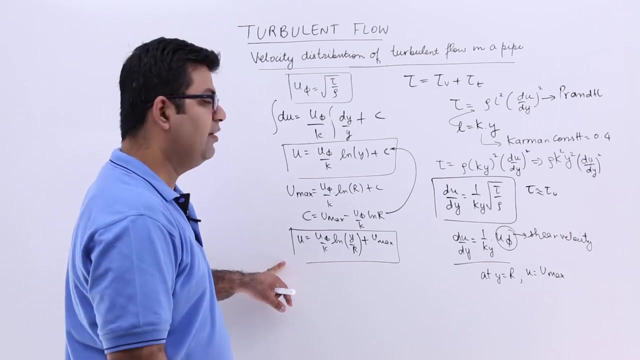 log r. So let's put the value of c over here, so the value of u will now become u. phi is equal. become u phi upon k into log. this will become y upon r. okay, plus this would be u max. this would be u max. so this is the equation that you get. so from here you can very well find.